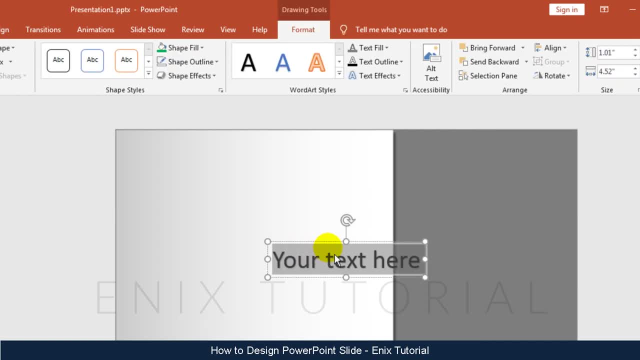 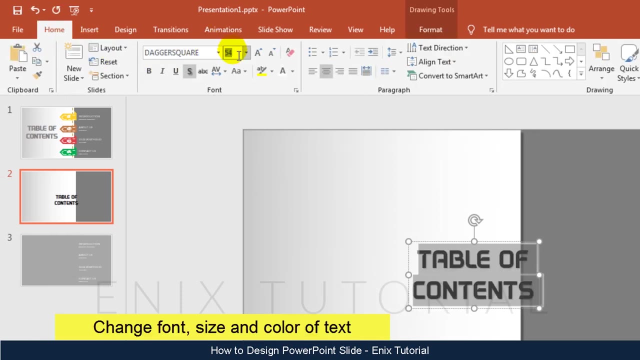 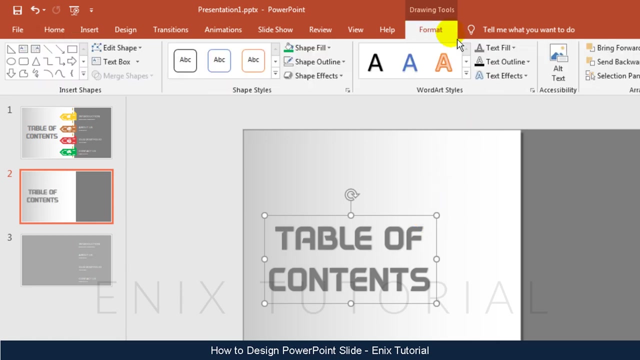 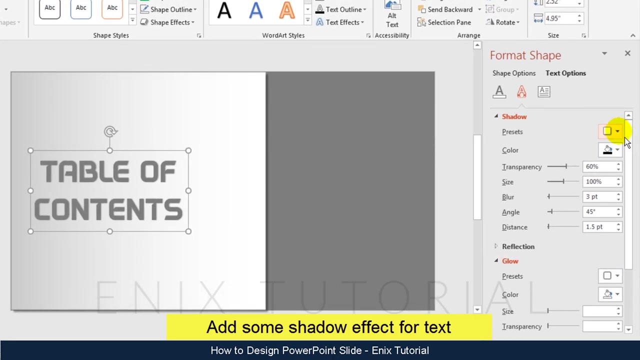 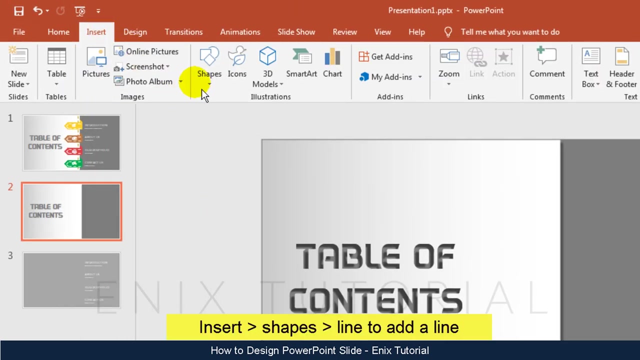 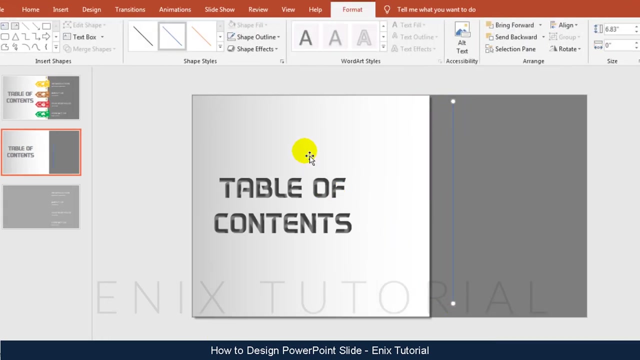 Then select all text box. Click word art to add text and title. Then change size, font and color of text. We'll see you next time. Go to Insert Menu Shapes. click Line to add a line. Then change color, thickness and dashes of line. 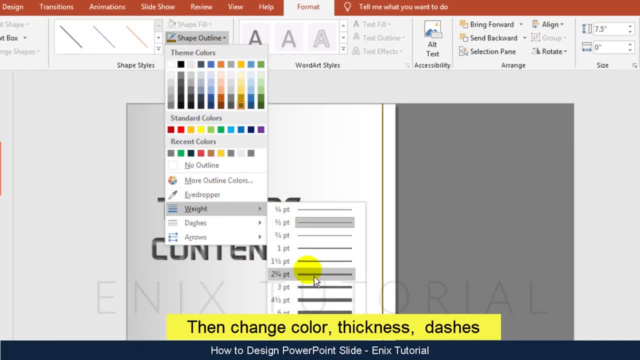 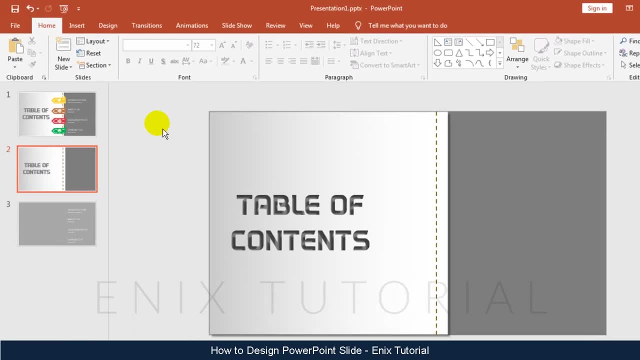 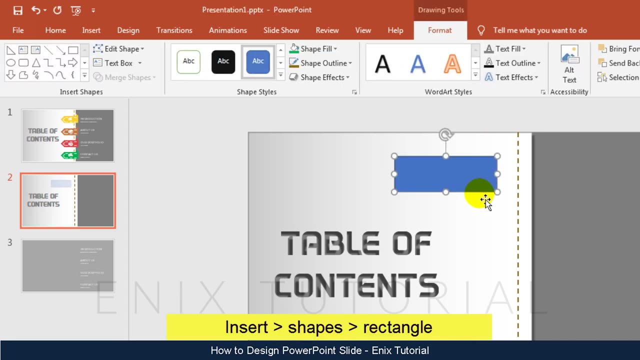 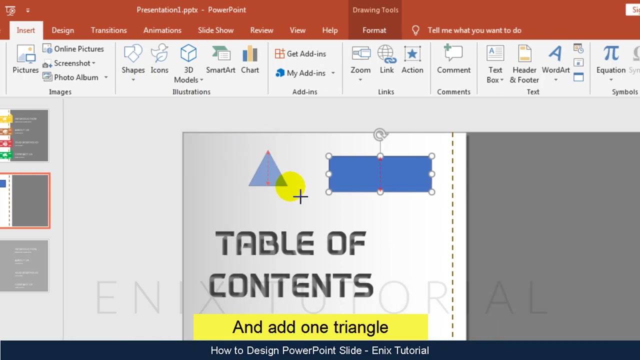 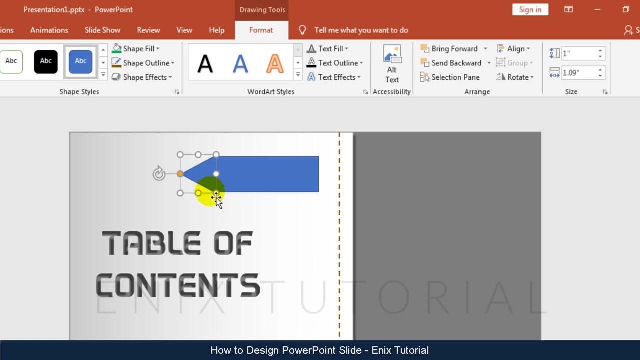 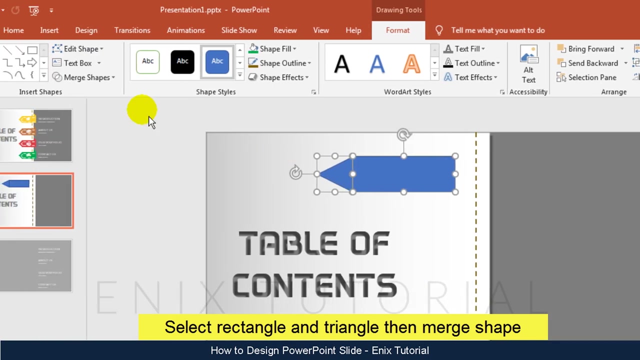 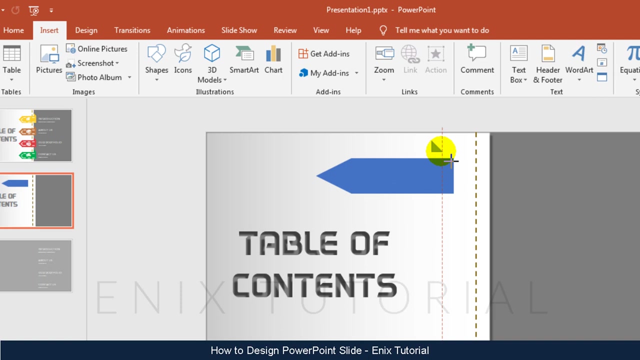 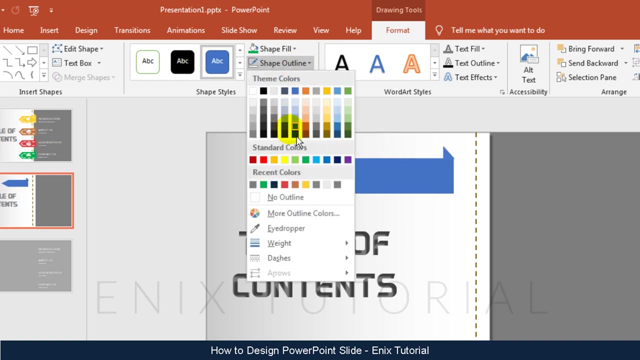 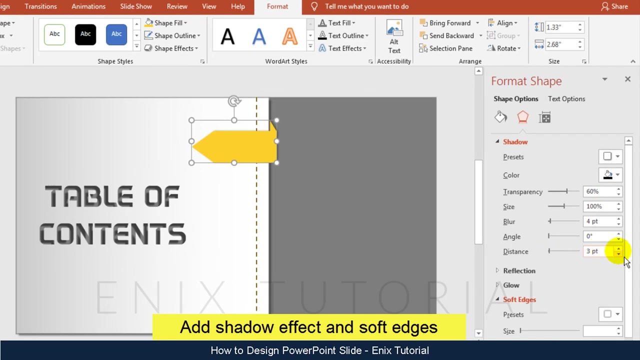 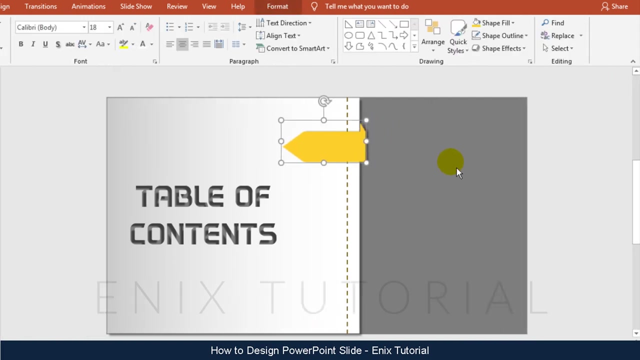 Insert Shapes, Rectangle, Draw a rectangle and one triangle. Select Rectangle and Triangle. then Merge Shape. Remove Shape Outline, Then resize and change color. I will change color of this shape And add shadow effect and soft edges. Insert Shapes and click Line to add a line. 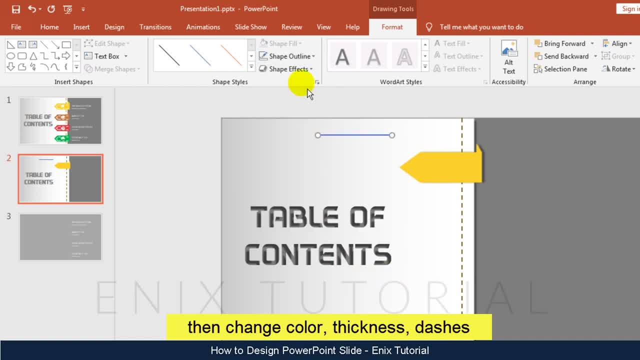 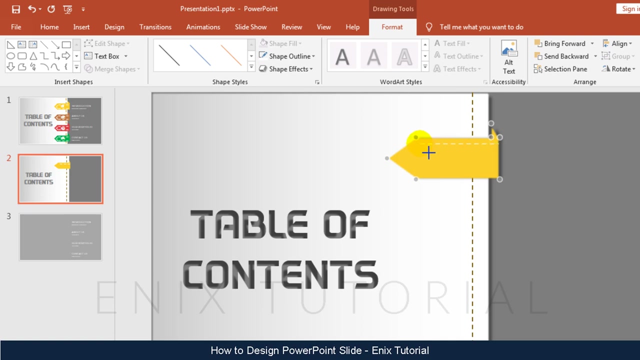 Change color, thickness and dashes, Then rotate over, Then say okay And you're done. This becomes the basic shape of the hands. In the next video, I will show you how to use恩ny bar. I hope you find this video useful. 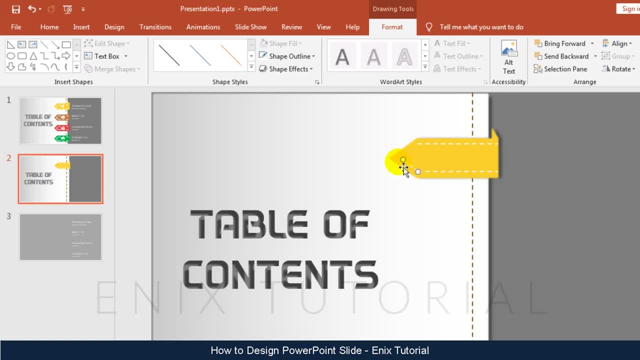 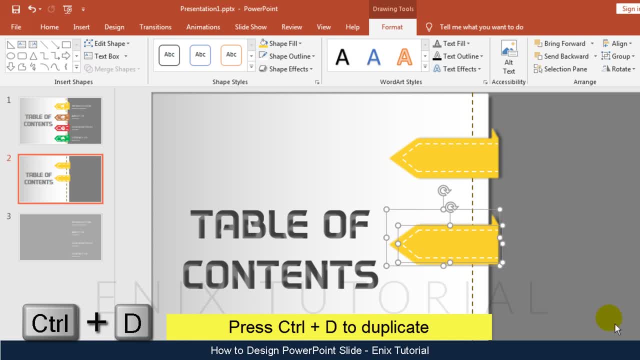 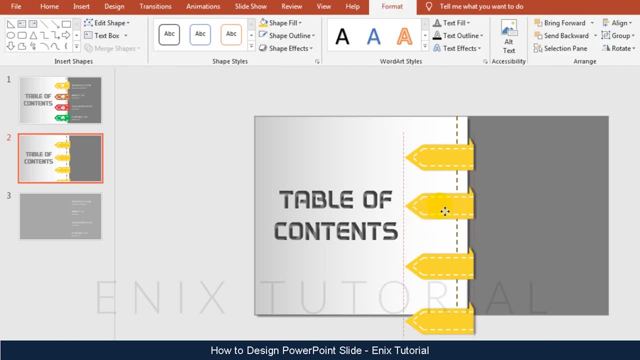 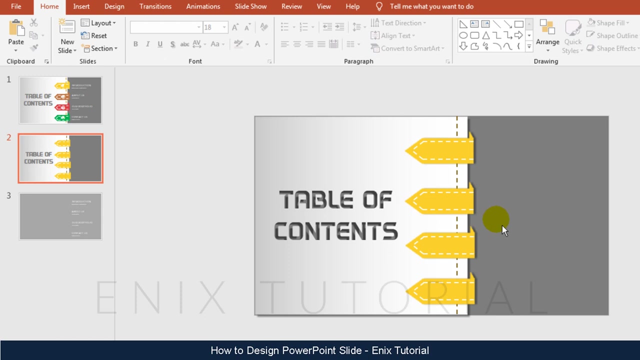 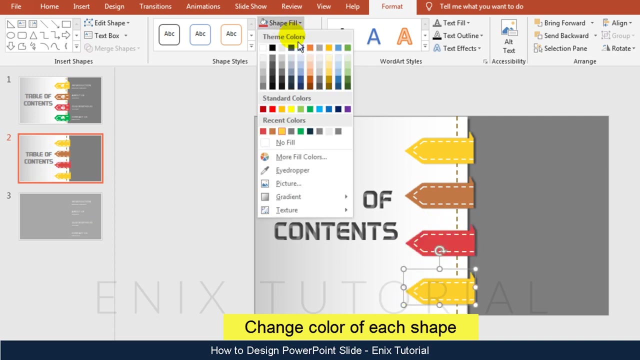 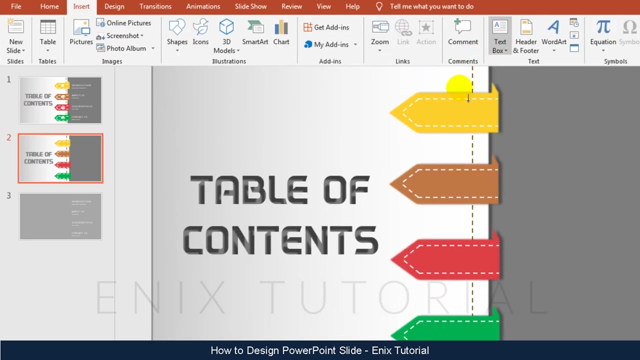 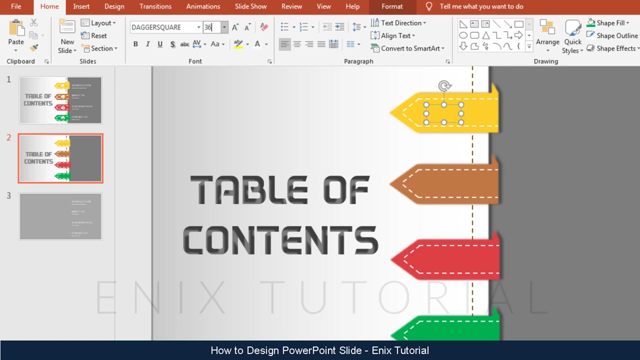 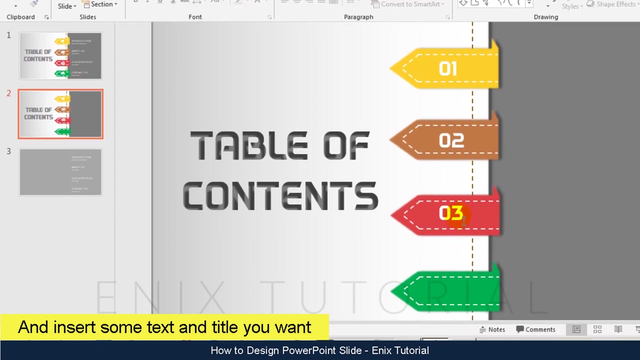 Adjust position of each shape. Then change color of each shape. Go to insert menu to insert text. I will add some number. Select the text. I will cut a couple lines. Then we need to edit this text. Let's see how our text will be. Let's do the same in the next picture.